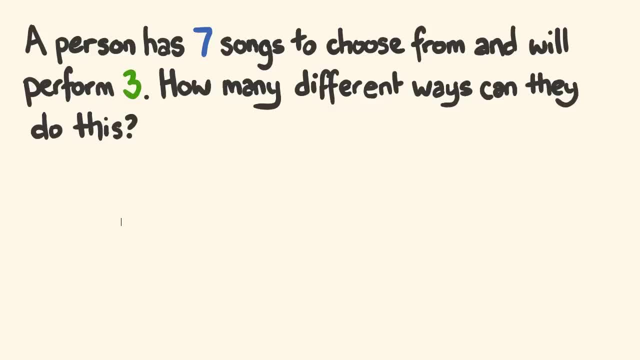 So question one: A person has seven songs to choose from and will perform three. How many different ways can they do this? So, for any of these questions, the very first thing you were to do is really identify it as a combinations question. 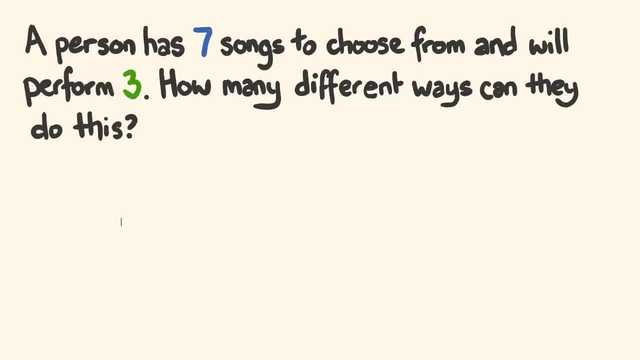 or a permutations question Once again, with combinations order doesn't matter. It's say like selecting three things from a bigger group but you don't really care what order they come out in. But with permutations order does matter. 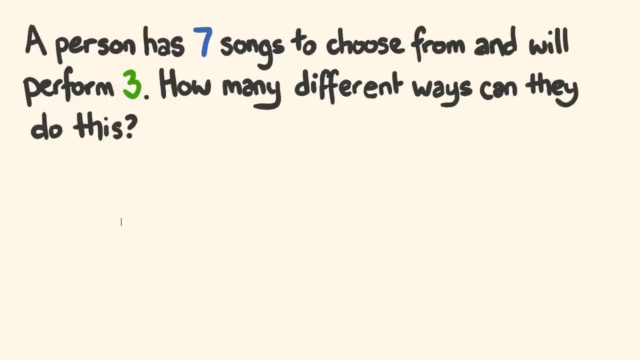 And with this particular question it is a permutations question, Order matters. There is a very definite first song, there is a very definite second song and there is a very definite third song. So the way I'd approach this particular question is as follows. 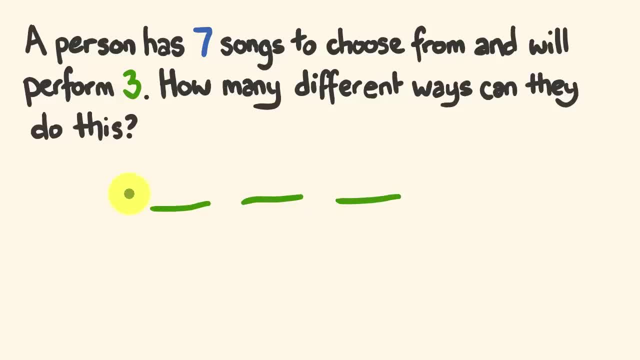 I would. I'd put three different spaces for the three different songs that are going to be sung And then I'd go: okay, for the first one, for the first particular song. how many choices does this person have? They have seven songs they can choose from. 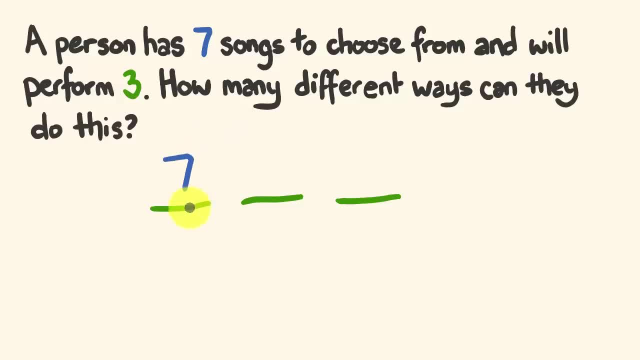 And then for the second song: well, they've already sung one of the songs in this space here, so now they've only got six spaces to choose from, six songs to choose from. And for the third song: well, they've already sung two songs now from the seven. 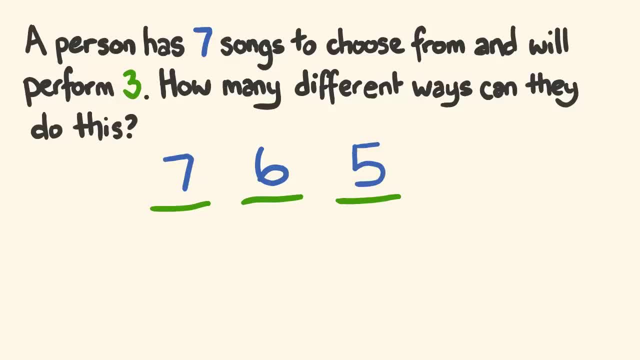 so now they only have five songs to choose from, And what we then did, What we then do, is we multiply this through and it will work out the number of different permutations. there are Seven times six times five is 210 different ways of selecting these songs. 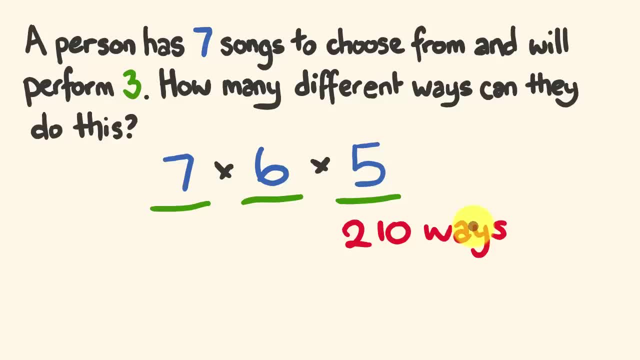 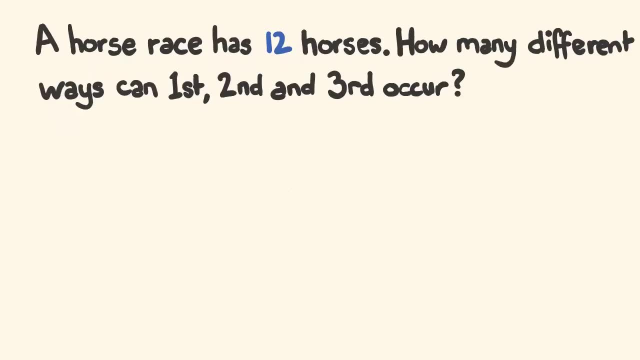 Okay, you might have used the rule for that and hopefully you would have got the same answer for that. Okay, but that's the way I attack these. We'll go to the second question, Question two. A horse race has 12 horses. 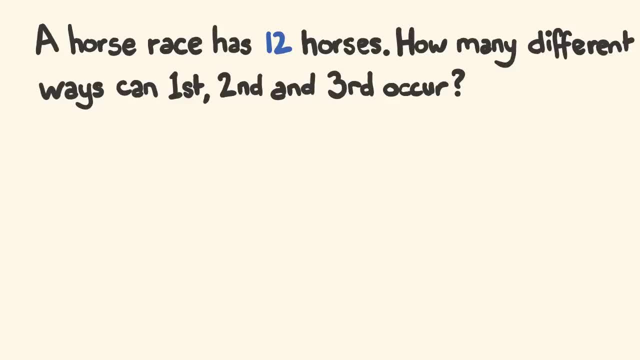 How many different ways is it? How many different ways is it? How can first, second, third occur? Okay, Now, once again, you're going to look at this and say, well, is this? In this question does order matter. 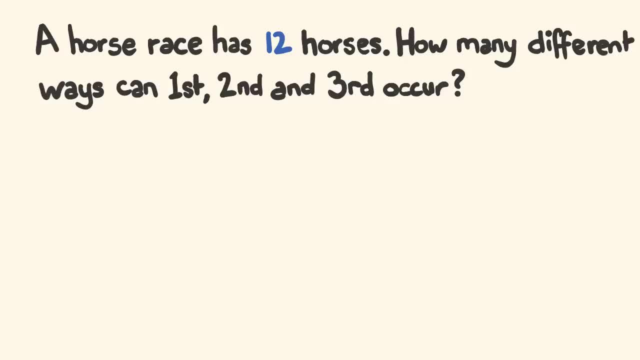 And I would say it very definitely does, because I've actually quite specifically stated: we've actually We want a first, a second and a third. Okay, So how would you do this? You give it a fly, You see it. 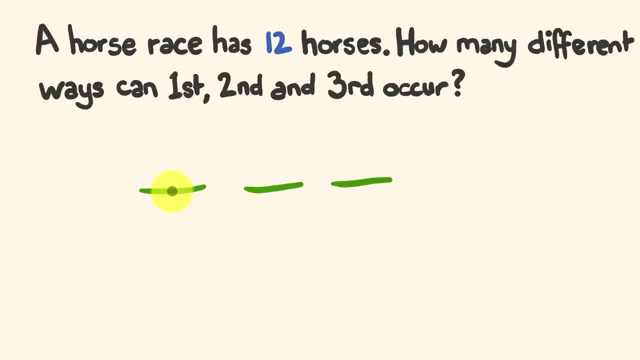 You give it a go, Okay, you select, You've got the three different spaces, the first, the second and the third, And for the first one you have 12 possibilities, 12 possibilities of which horse might come first. 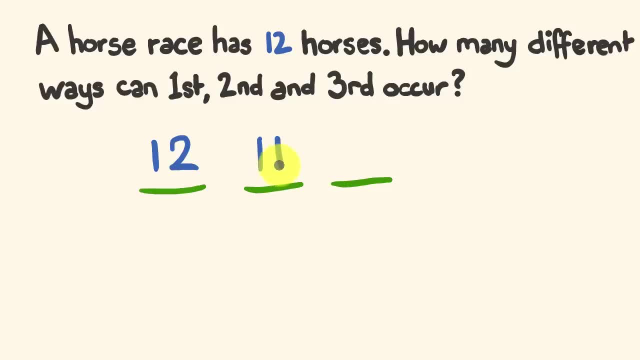 But once that horse has come first, then you're left with 11 different possibilities for second, And then for third. then you're only left with 10 different possibilities. Okay, So what would you do then? You would multiply this through. 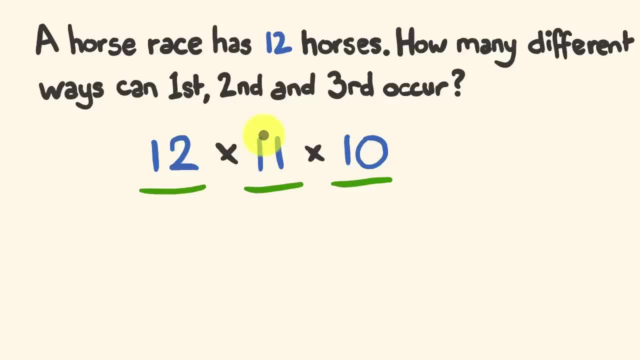 12 times 11 times 10.. So 12 x 11 is 132, times 10, the answer's going to be 1,320.. Different ways of doing this, Okay, But I'm just going to take this a little bit of a further step. 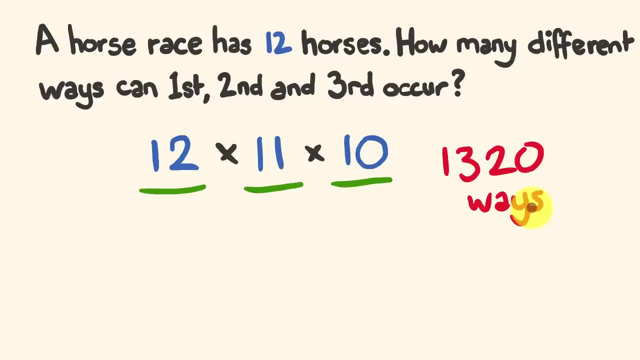 What if order didn't matter? What if we were just saying: how many different ways can we say what the first three horses will be, without actually really caring whether they're first, second or third? Well, we take this a little step further. 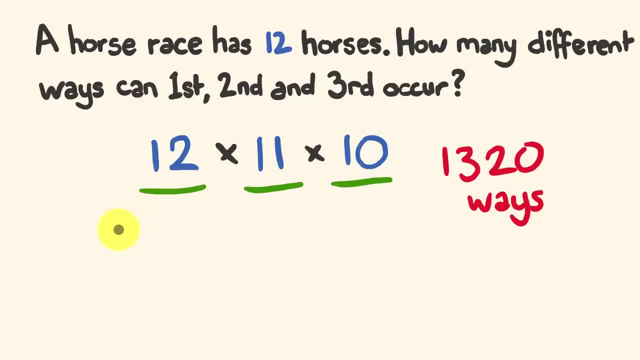 It would become a combinations question then, And then what would happen is we would say: well, okay, there's one, two, three different places here, And that means there is three factorial ways of arranging these places. So we divide these out. 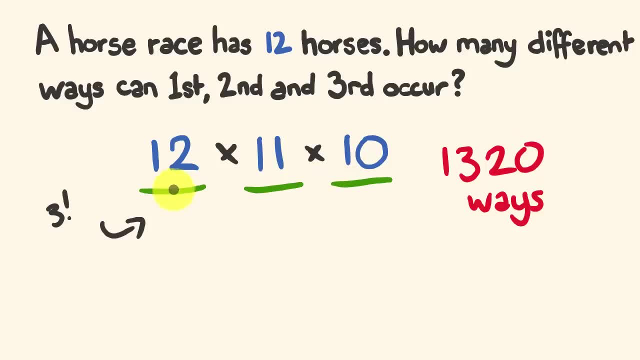 And that's how we do combinations- is we divide it by the number of places. here factorialized Three factorial is 3 x 2 x 1, which is equal to 6.. So we're going to end up with 1320 over 6, which is going to be equal to 220 different ways. 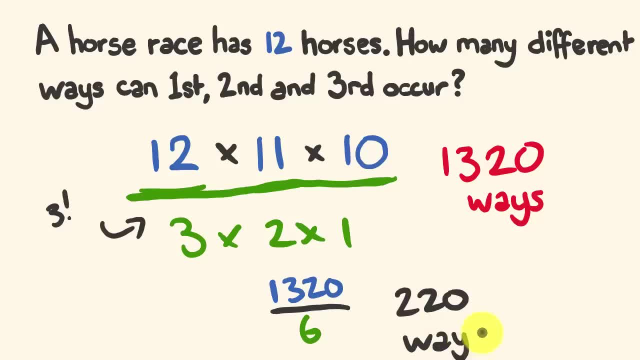 And that's if order doesn't matter. Okay, And that's it. Extra step we take if we're doing combinations questions. This is if you were just working out the permutations and order did matter. This is if you were working out the number of different combinations and order didn't matter. 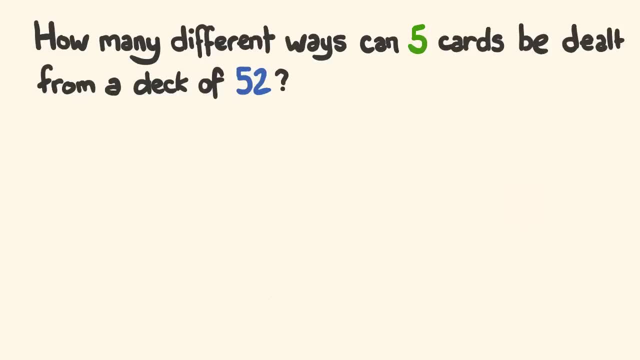 So we'll go to a different question now, Question 3.. How many different ways can five cards be dealt from a deck of 52 cards? Okay, Now with this particular question, does order matter? No, it doesn't, Because you know, the card that got dealt first could be dealt fourth. 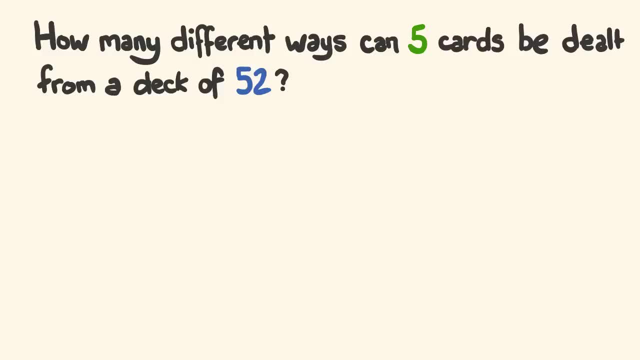 So this is a combinations question, So we're going to treat it like this. We did that last part of that question we did just before. I'm going to get the five spaces- the 1,, 2,, 3,, 4, 5- for the five cards. 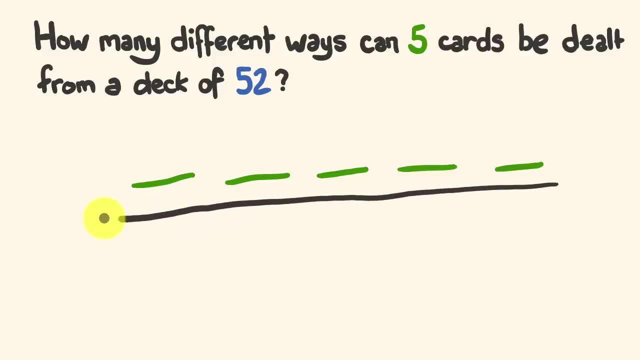 But then I'm going to divide it by the number of different ways that these five cards can be arranged. This is the same as 5 factorial, 5 x 4 x 3 x 2 x 1.. So for the very first up top here, how many different ways can 52 cards? 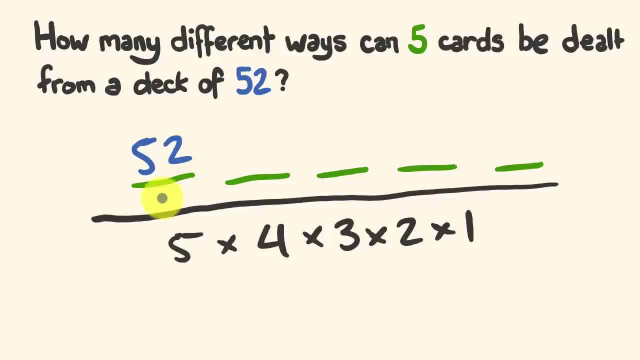 these be picked out. Well, the first one: we have 52 cards to choose from. The second one: we have 51 cards to choose from. The third card selection: now we have 50 cards to choose from. The next card: now we have 49 cards to choose from. 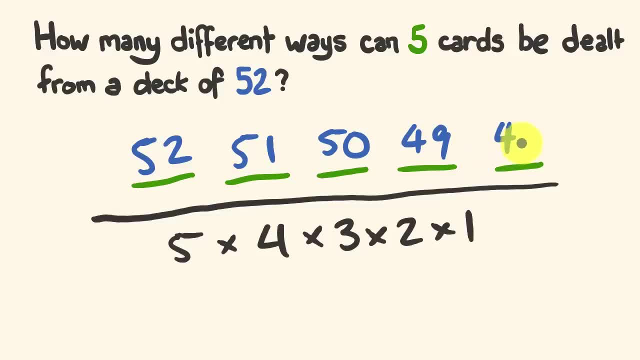 And the next card now, because we've already chosen these ones. we have 48 cards And then we'd multiply these through And you can imagine you're going to get a pretty big number when you do this. The number of different possibilities is 2,598,000. 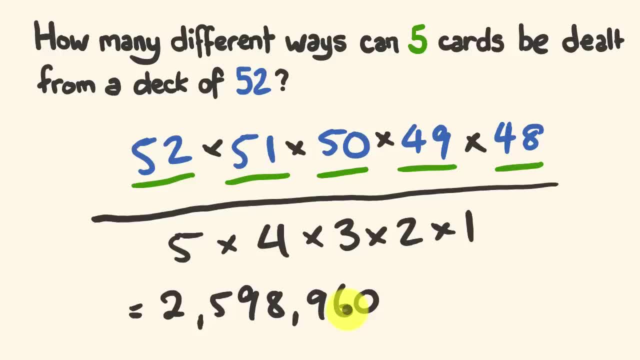 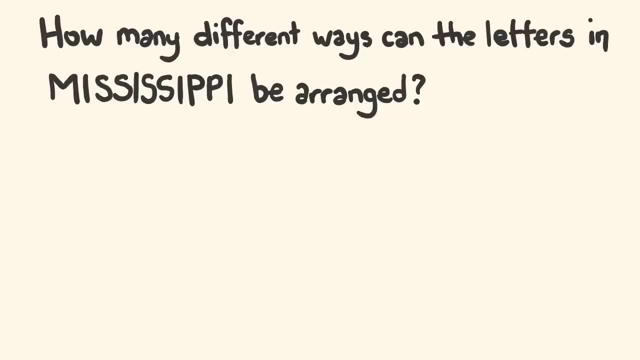 1,960.. Okay, Okay, question four: How many different ways can the letters in the word Mississippi be arranged? Now this straightaway you're going to look at and say, is this a combinations or a permutations question? And you'll probably think order does matter in this. 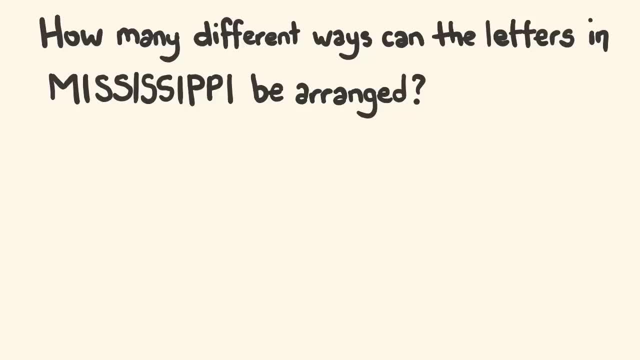 Order definitely matters. It's all about actually arranging things in a particular order. So it's a permutations question. But it's a bit of a special question because it's not just a matter of arranging 11 different ways. So we're going to look at the letters which there are in the word Mississippi, because we have these repeats. 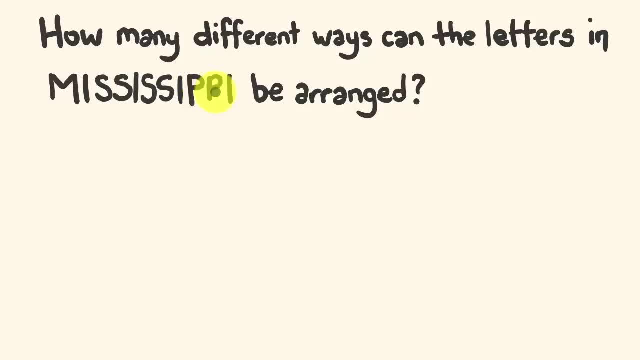 If you were to change the position of these P's, they're not going to change the actual words, So we've got to take into account these particular repeats. So the way that we do this is as follows: First off, the number of different ways that these letters Mississippi could be arranged is 11. factorial: 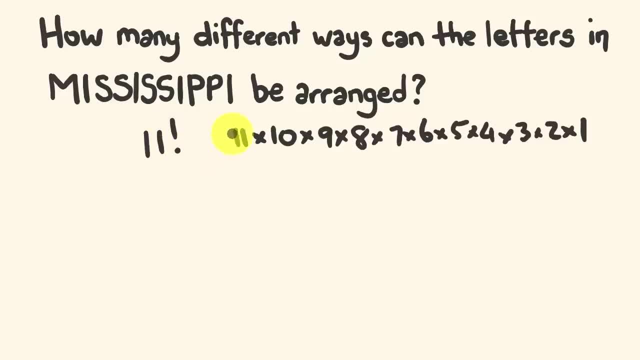 Okay, So 11 factorial, which means this Times 10, times 9, times 8, times 7, times 6, times 5, times 4, times 3, times 2, times 1.. 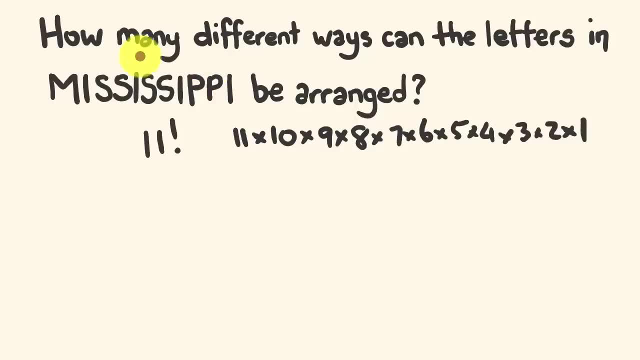 But to take into account the repeats, we just count the number of repeats for the different letters. So for the letter P, there is 2 of them, For the letter S, there is 4 of these, And for the letter I, there is 4 of these. 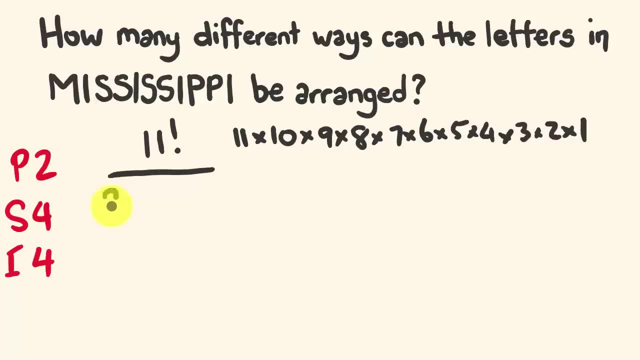 And we divide these out as follows. So we're going to divide by 2 factorial, 4 factorial, 4 factorial. So we get something that looked like this: And now what we could do is we could start counselling things out: This 4, 3, 2, 1, and this 4, 3, 2, 1.. 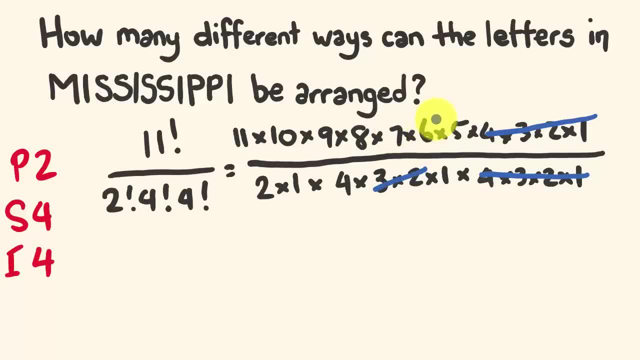 And you might say: okay, this 3 and 2 here is equal to 6.. And we have a 4 and a 2, which is equal to 8. So we're left with 11 times 10, times 9, times 7, times 5.. 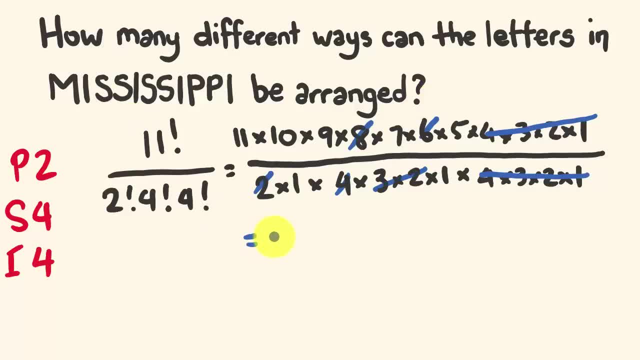 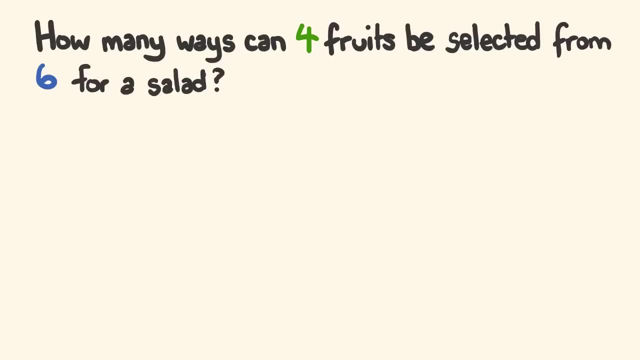 This is equal to 34,650 different words, And that's the way you do these types of questions, okay, You just divide by the repeats: factorialised Question 5.. How many ways can 4 fruits be selected from 6 for a salad? 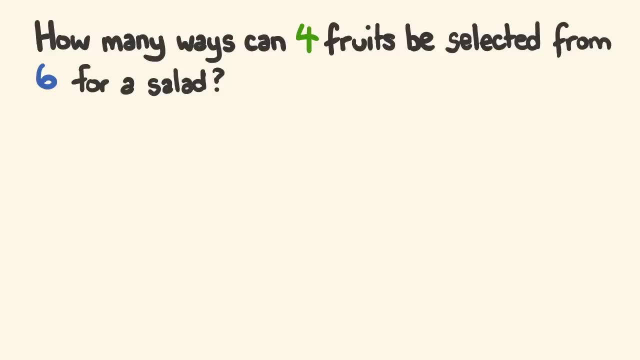 Nice, easy question. Does the order matter? Hey, no, it doesn't. This is a combinations question. This is a really, really nice, easy question, this one. So I'm going to draw the 4 spaces for our fruits: 1,, 2,, 3,, 4.. 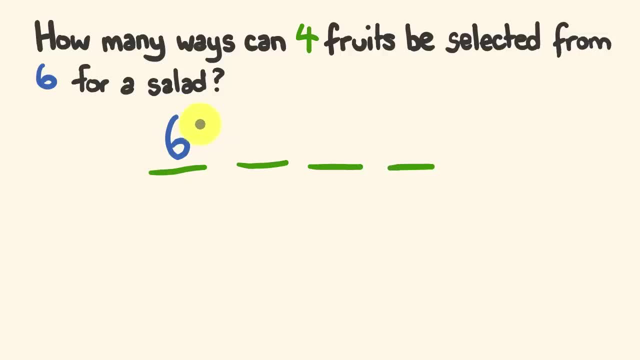 And so for the first fruit, we have 6 to choose from, And now we've already chosen that particular fruit. Now we have 5 for the second one. 5 for the second one we're going to select. And then for the third fruit we're going to select. 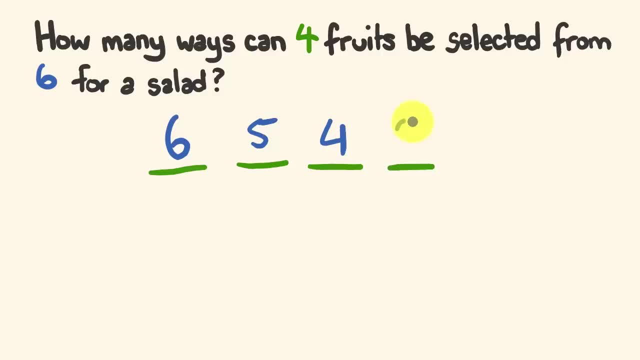 We've already selected 2 out of the 6, so we're left with 4.. And for the next one we're left with 3.. And we're going to multiply this through. But with all combinations we have to divide. 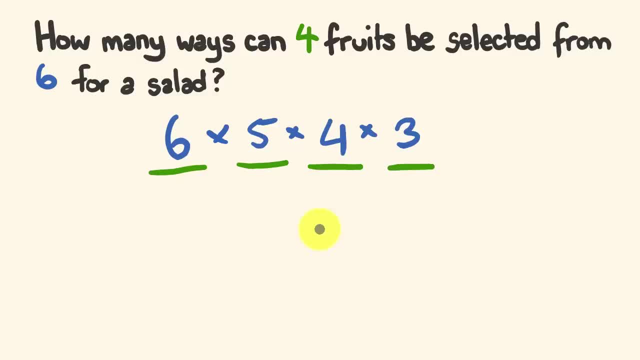 Because we're going to have to take into account the order doesn't matter. We're going to divide by the number of different ways these 4 objects can be arranged, also To get rid of those particular arrangements: 4, 3, 2, 1.. 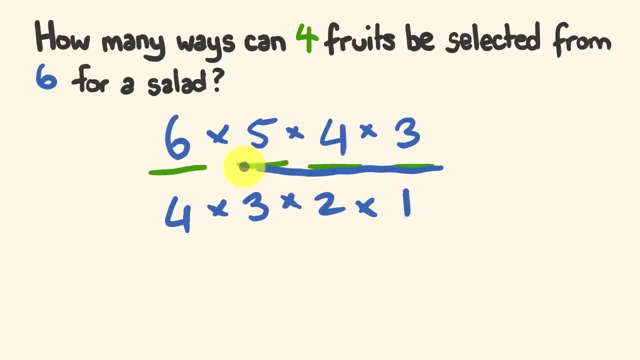 Multiplied And that's what we're left with, So we can cancel out once again. This 4 is going to cancel this 4 out. 6 is going to be cancelled out by the 3 and the 2.. 3 times 2 is 6.. 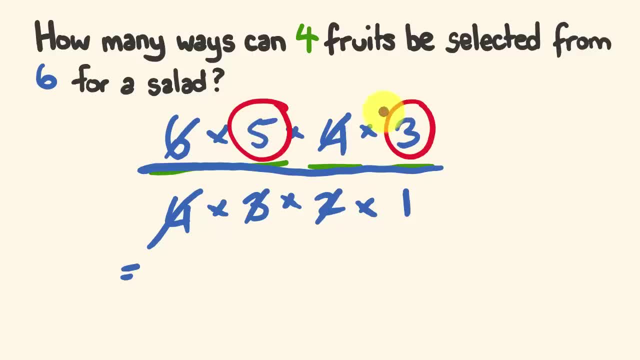 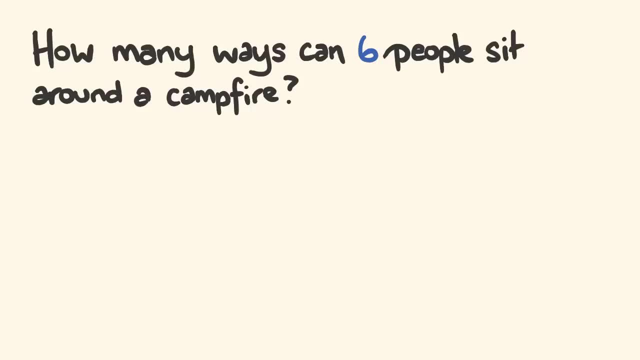 And we're left with 5 times 3. Which is equal to 15 different ways. So for the sixth question: How many different ways can 6 people sit around a campfire? Does all of it matter in this question? You might look at it and say, hey, it definitely does. 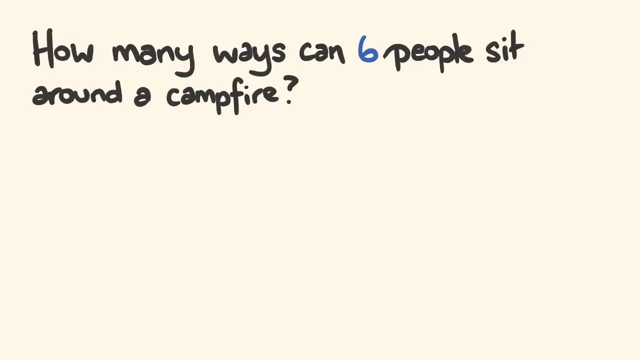 It definitely does. So this is a permutations question. Okay, But it's a special type of permutations question Because if I was to draw this campfire, And I'll draw the 6 people sitting around it- 1,, 2,, 3,, 4,, 5,, 6.. 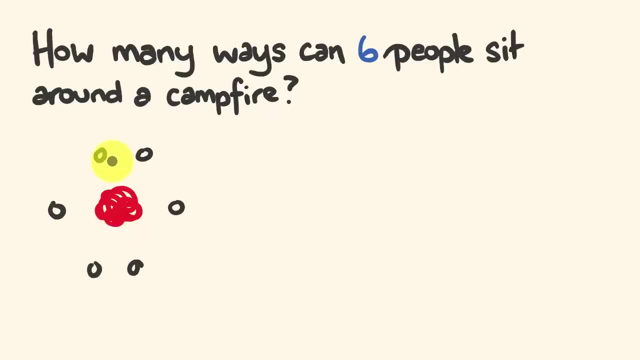 And you're going to realize that these people are sitting in a circle, And so, for this particular question or these particular questions, I'm going to consider that if everybody was to get up And move counterclockwise this way- And I'll look at one person in particular- 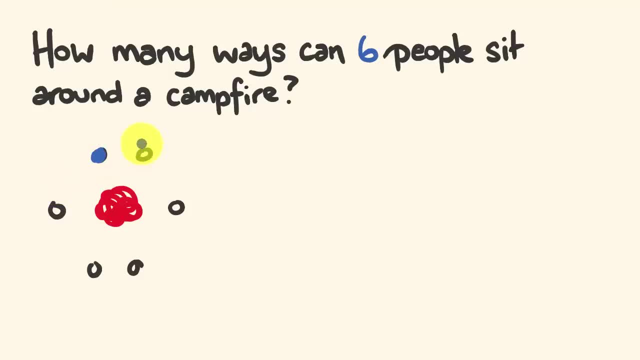 But you're going to assume that everybody's following his lead. So this person will go to where he is And this person will go to where he is And this person will go to where he is. You're going to notice that We're going to assume that these are actually moving to a similar sort of arrangement. 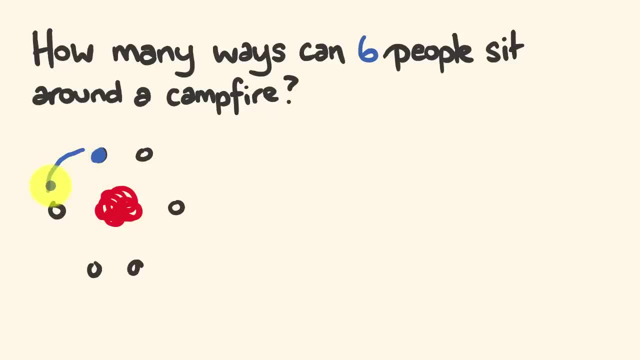 Okay. So if this person was to move this way, We'd have one similar arrangement. Or if they were to move to this way, We could have another similar arrangement. Or if they were all to get up and now move counterclockwise this way. 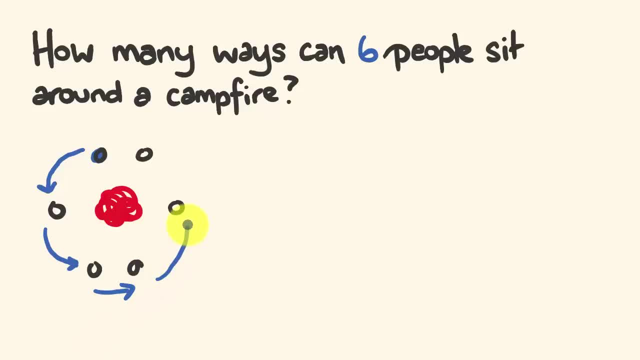 They'd still all be relative the same way. Or if they were to move this way, We'd have a similar arrangement again. Or if they were to get up and move counterclockwise once again, They'd have a similar arrangement. Back to the same position. 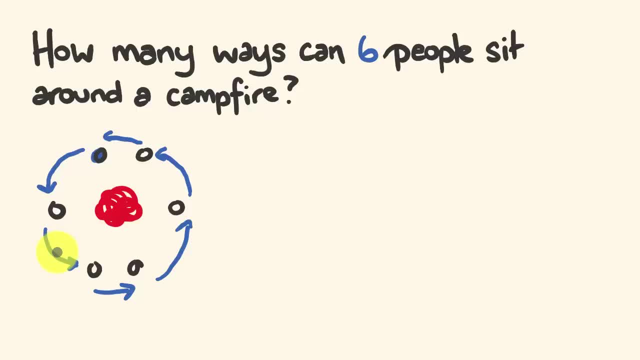 We have 1,, 2,, 3,, 4,, 5,, 6. Similar arrangements that we have to take into account. So we're going to divide out by those. Okay, So we're going to divide our answer by 6.. 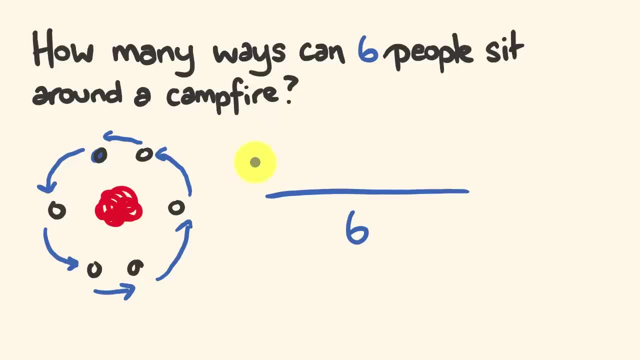 So 6 different people, If they were in a line, could sit together 6 times, 5 times 4 times, 3 times, 2 times 1.. Different ways, But these are going to cancel each other out, So we're just left with 5 times 4 times 3 times, 2 times 1..